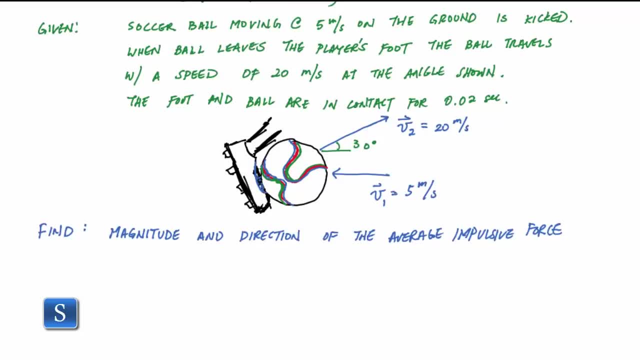 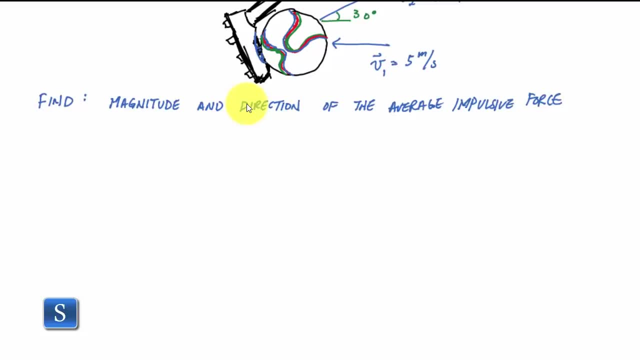 the principle of linear impulse and momentum. let's just make sure that we're all on the same page here. i'm going to write out this principle real fast and the idea in most textbooks. what you'll see is that the momentum at one plus the sum of all the impulses, which is this integral. 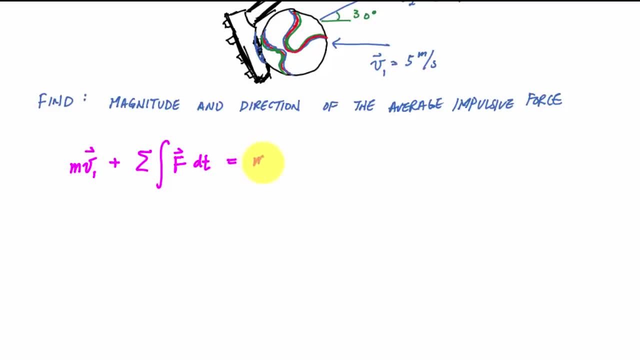 of fdt is equal to the momentum at two, And it's important to note this is a vector equation. So what we can do with this vector equation is break it up into components, depending on the coordinate system that I'm using. So you might break this equation up into X, Y and Z components. So what you really 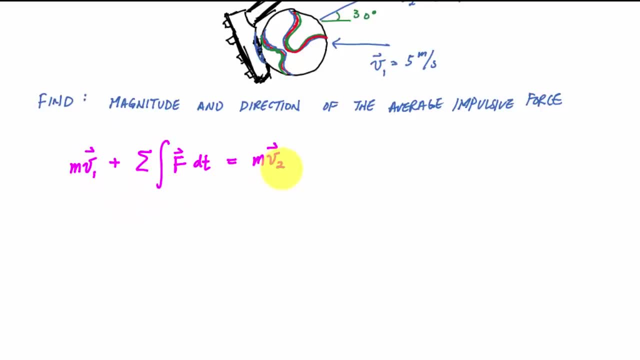 see here. in 2D would be two equations and in 3D three possible equations. Another way that I like to look at it is that, you know, I have a particle that has a state of momentum, and then all these 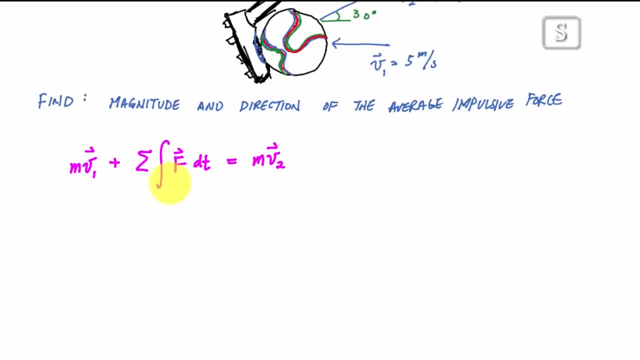 external forces or impulses are applied And really it's like a force for a certain specific duration of time, you know, and I always think of like a punch. When you punch something, it makes contact for maybe a split second or so. it imparts a force or an impulse and it changes the momentum. 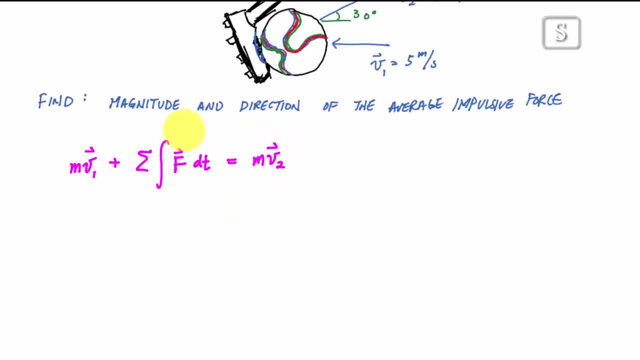 or the direction, And so the first thing I'll do for this problem when I apply this is: I like to draw the schematic of the particle that I'm looking at. In this case, it would be this soccer ball. What I want to do is draw a schematic that matches. 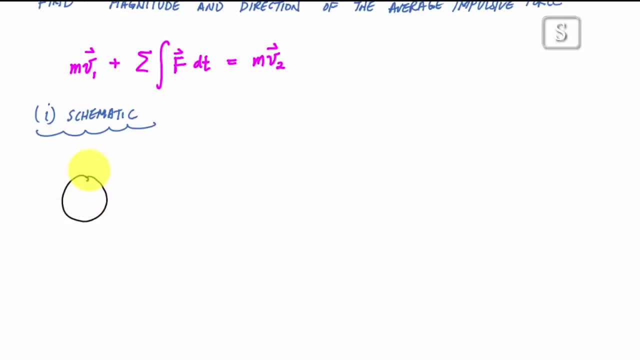 This is my equation. Initially, I have my soccer ball here. It has a velocity towards the left plus the impulse that this particle receives, which is some force from my foot here, this F for a certain duration of time. So I'm going to call this F D T, and it has an unknown angle which I will just call. 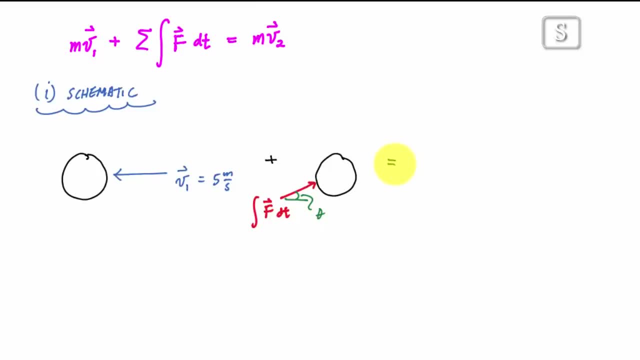 beta, And after that kick or that contact with my foot, the soccer ball will have a velocity of 20 meters per second. That's an angle of 30 degrees, And I know what the mass of my, my soccer ball is. I do know And you know. 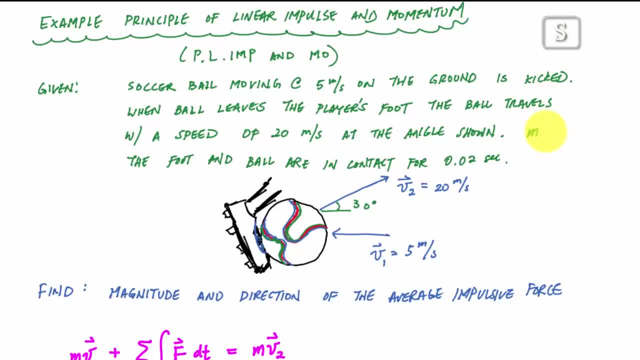 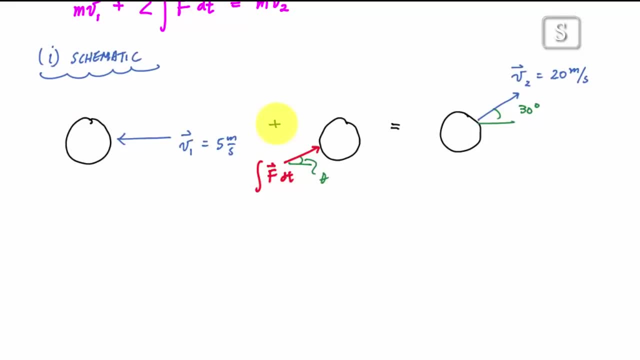 looking at FIFA and the, the mass of the soccer ball that I'm using is 0.43 kilograms. All right, So I have my schematic that looks like my equation. I know the mass of my soccer ball. Here's my momentum at one, the impulse, and then my momentum at two, And I'm going to say: I'm going to. 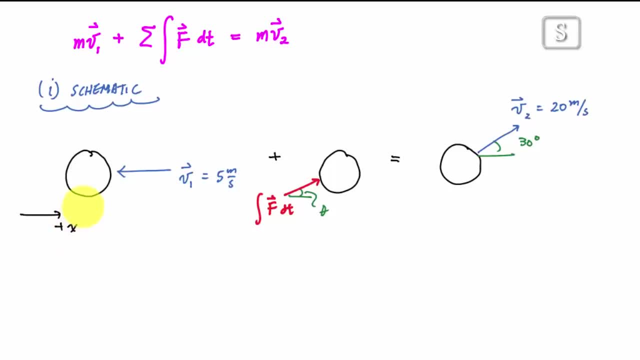 establish a coordinate system. I'm going to say: this is my positive X direction, or my positive horizontal, and my positive vertical direction is upwards, And so now I'm just going to go ahead and apply the principle of linear impulse and momentum, or P, L, I, M, P and L? O, in each component. 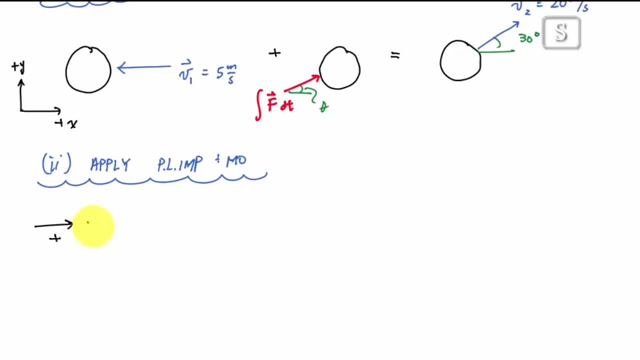 So I'll start with the horizontal direction and I'll say positives to the right. And so here my momentum in the horizontal direction, for here M one, M V one, which is to be the mass of the soccer ball V one. And this is negative because my 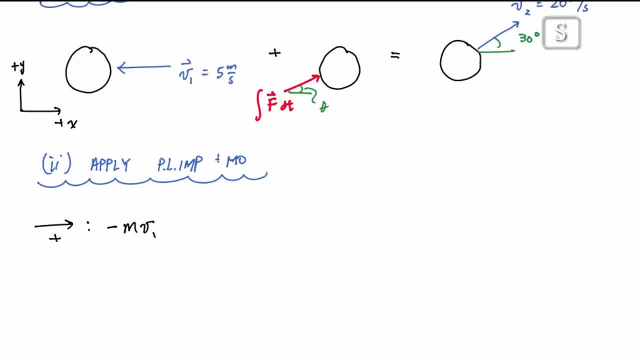 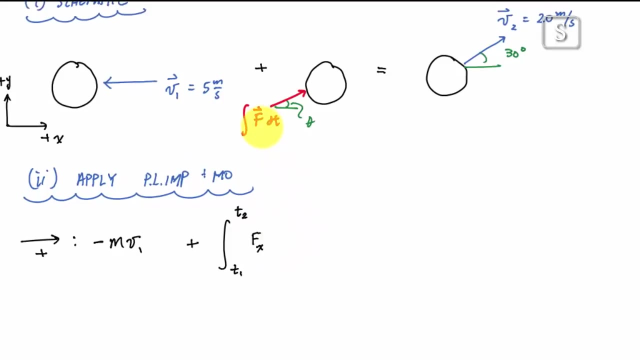 velocity is pointing towards the left with a magnitude of five meters per second. Plus, I would have the impulse from times T1 to T to the force of that impulse, D, T, And the horizontal component of this force would be the X component of this force here. 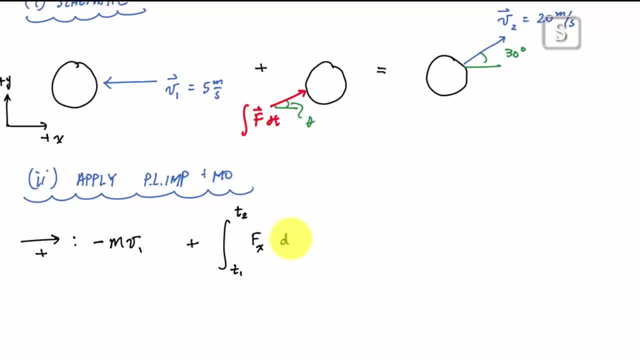 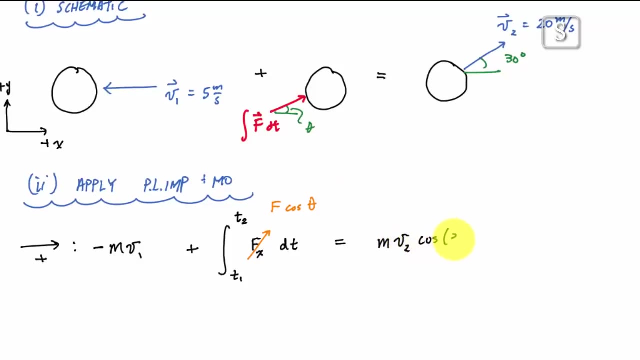 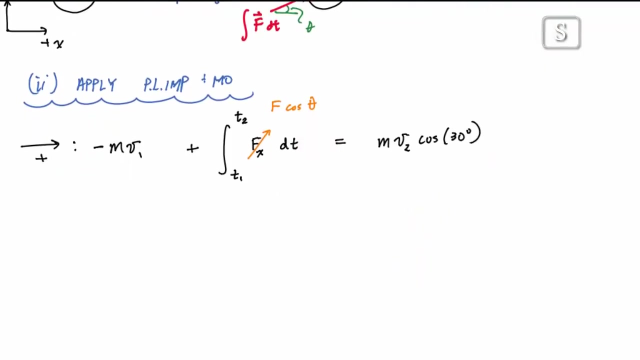 And that would be FX, D T, and really FX is just F cosine of theta, And this is equal to my horizontal of momentum at stage 2, which would be m v2 cosine of 30 degrees. and it's positive because my horizontal component is going to the right. and now I write my vertical component equation, my 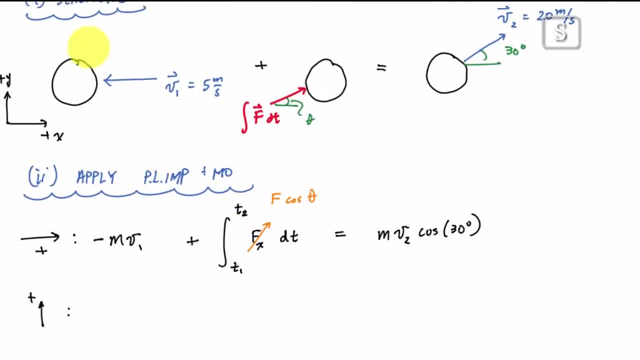 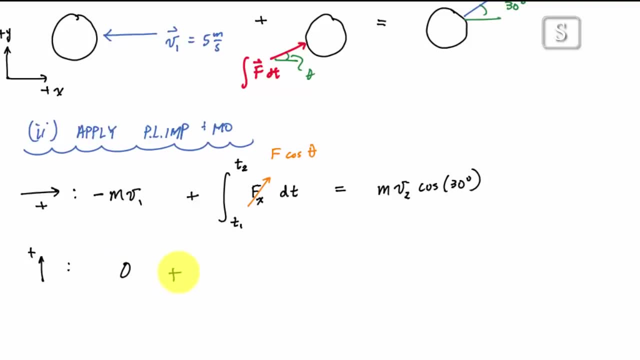 vertical positive. I have no velocity in the vertical direction, so no momentum in the vertical direction here at stage 1, if you will. so that's just 0, plus I would have here t1, the t2, f, the y component of this force, dt, which would just be f sine theta. and again, it's positive because I'm 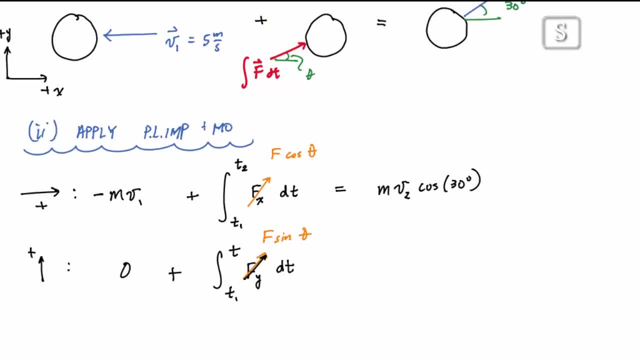 assuming that it's pointing upwards- is equal to m v2 sine of 30 degrees. and the way I've set this up, I have. I know the mass, I know the velocity at 1, I know the mass and the velocity at 2, boom, boom. so my only two unknowns are the magnitude of the force and this. 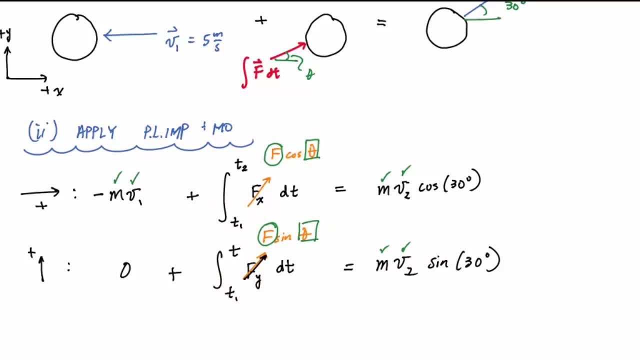 angle theta and really I know the time t1 to t2 because the total duration of time is 0.02 seconds. what I'm assuming here is that this force is constant and not dependent of time, because I'm taking an average value of the impulse. so this force, again, is not dependent on time. here, time t1 is the point. 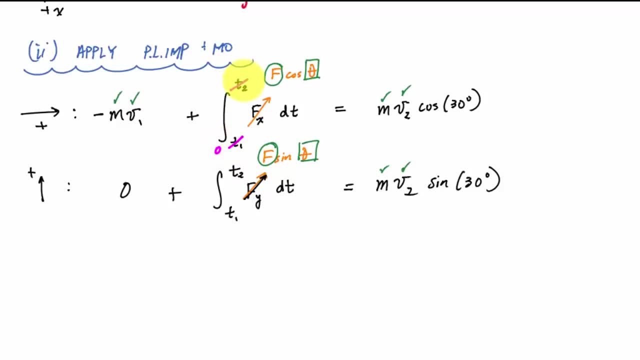 when my, when my foot just makes contact, so I'll call that zero, and then when my foot leaves the ball, it's 0.02 seconds, and same here: 0 and 0.02 seconds. so again I'm left with two equations, two unknowns. all I got to do is 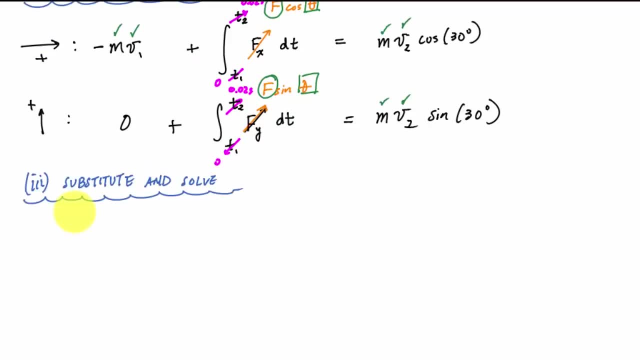 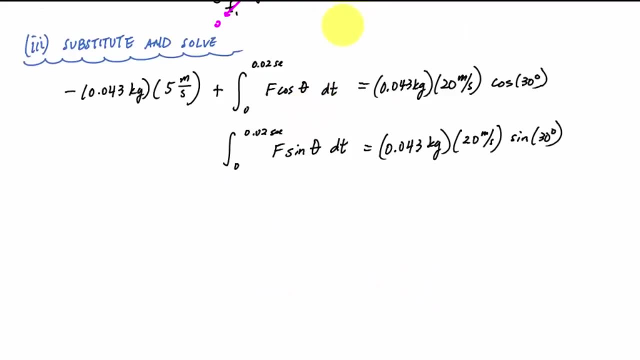 substitute and solve. so I'm just going to plug and chug numbers into each equation. here we're assuming for the shape of this force function as a function of time. we're just assuming that the impulse term looks like this and this integral here represents the area. 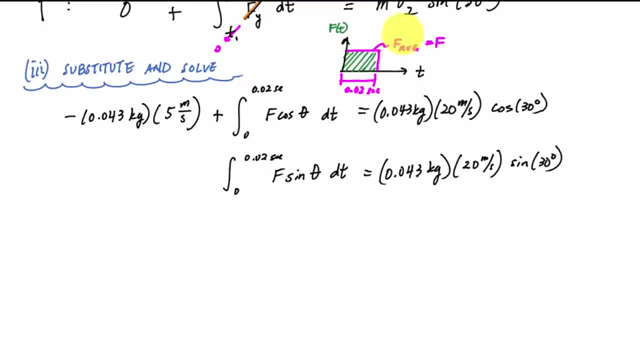 under the force, and this is that area is called the impulse, because this is constant. here, this force is it. we're taking the average value, so we're assuming it's constant, it's independent of time, and when I do this integral it's a pretty straightforward, and now all I gotta do is solve two. 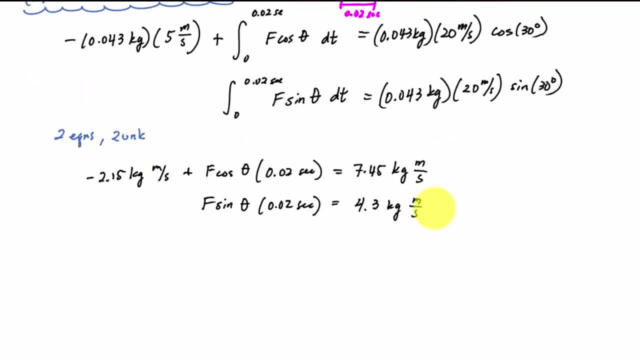 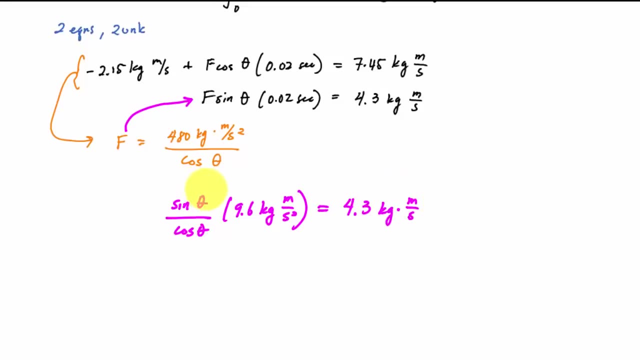 equations and two unknowns. so from this equation I get that F is equal to: and if I take this and I substitute this into the second equation, here I will get and here know that this sine theta, cos theta, that is just tangent theta. And if I take the inverse, 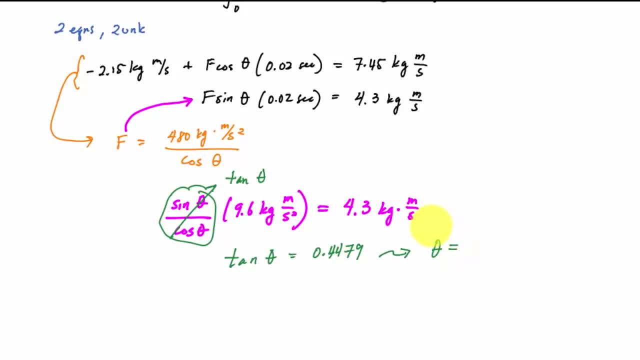 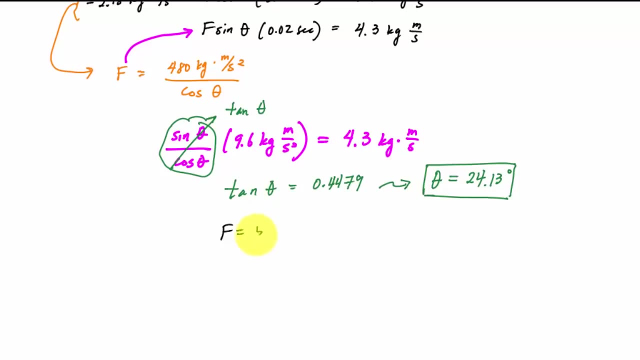 tangent. this will tell me that theta, the angle at which the ball is being kicked with that force, is 24.13 degrees. And I can just take this theta, plug it back into this equation over here, into one of the equations, and I can find my force: It's 525.95 newtons.